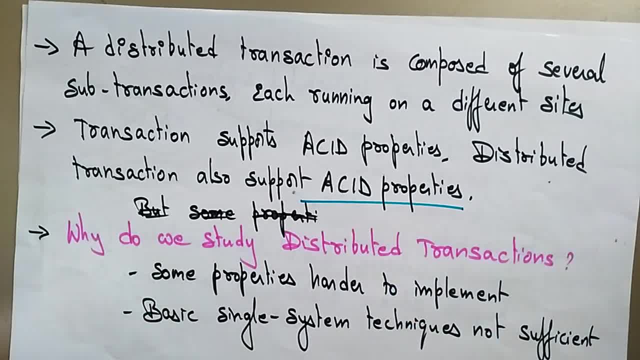 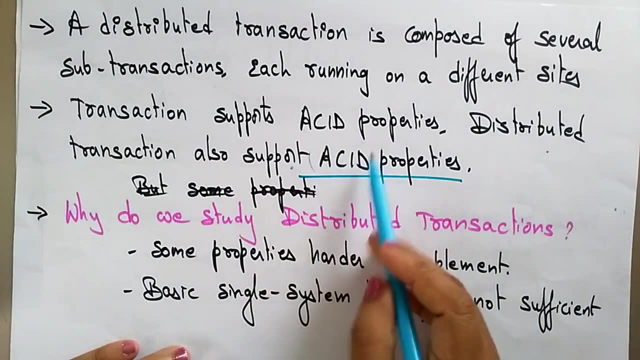 supports similar ACID properties, Then why we have named it as distributed transaction. Why do we study the distributed transactions? If ACID properties are there, then why we are also studying the distributed transactions? Because some properties are harder to implement in the acid: the atomicity, consistency, integrity and durability. so these are the different properties. 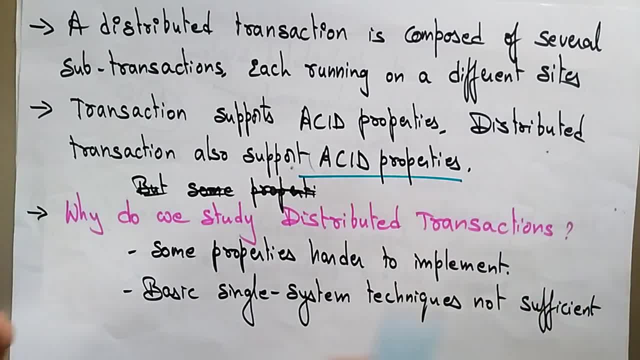 so in this some properties are harder to implement and the basic single system technique is not sufficient. in the centralized we are using only the single system techniques. one is acting as a coordinator. with the help of that coordinator everything will be sanding. so the main so here. 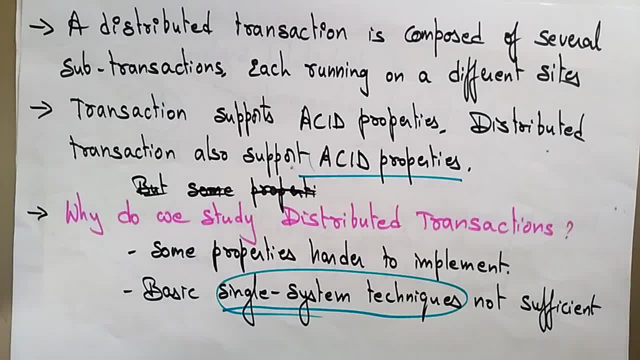 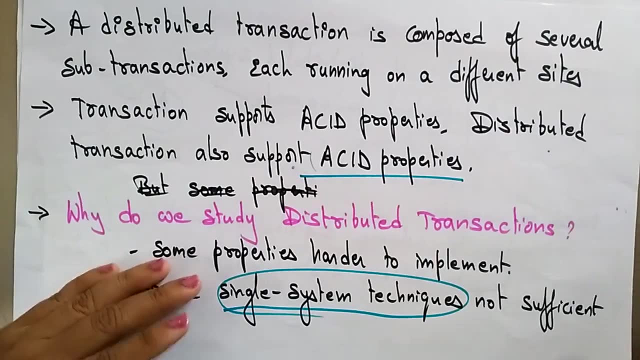 in the basic, the basic single core technique is not sufficient in for the distributed transaction. so that's why we are taking the distributed transaction to maintain these properties which are hard to implement it. so to maintain those properties and to work on the distributed environment, we are using the distributed transactions. so that is thing. so in the 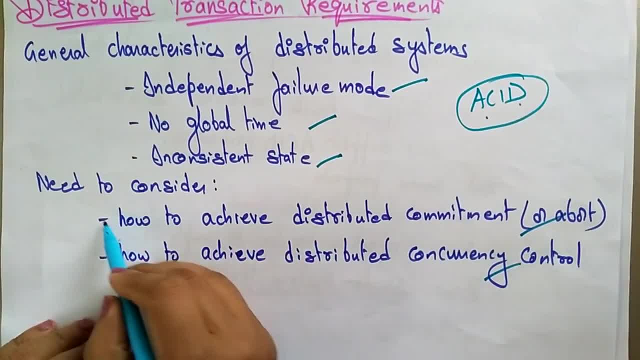 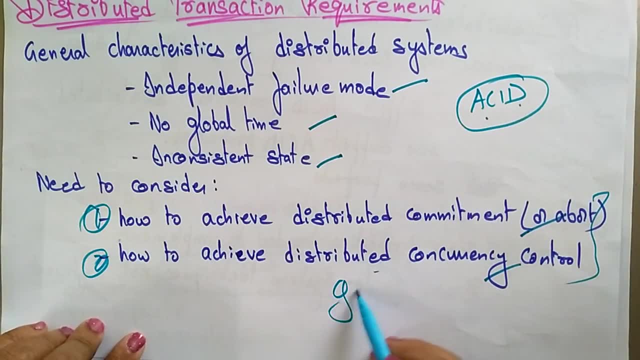 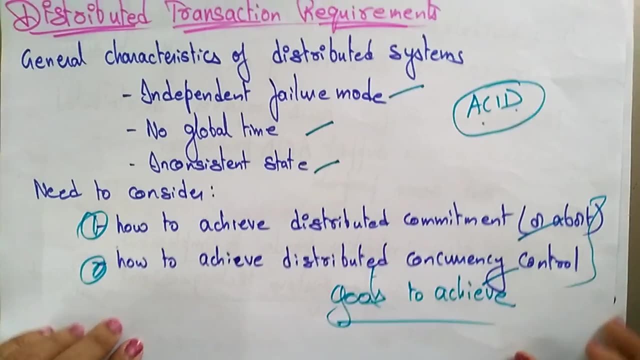 distributed transaction. we need to consider how to achieve the distributed commitment or abort, and how to achieve the distributed concurrency control. so these are all the two goals that we need to be find out. what is the goal to achieve. these are the two goals that we need to achieve in the distributed 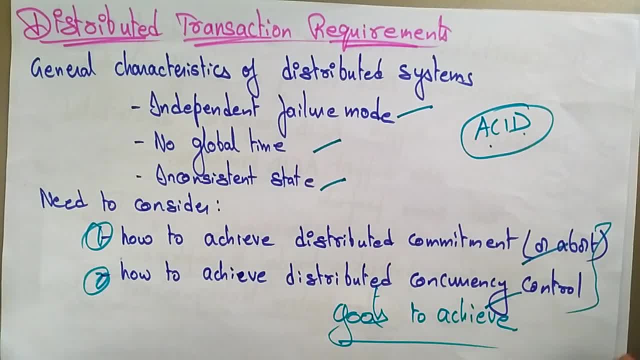 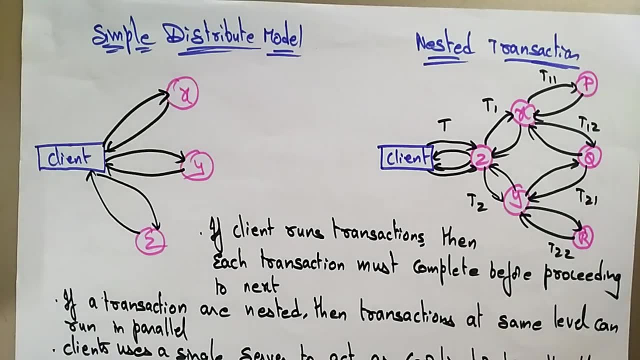 transaction, how to achieve the distributed commitment and how to achieve the distributed concurrency. ok, so before seeing how to achieve the distributed commitment and the concurrency, let me explain you a simple distribution model. in this simple distributed model and the, if you take the nested transactions, so here is the client, is there and so many other processes. 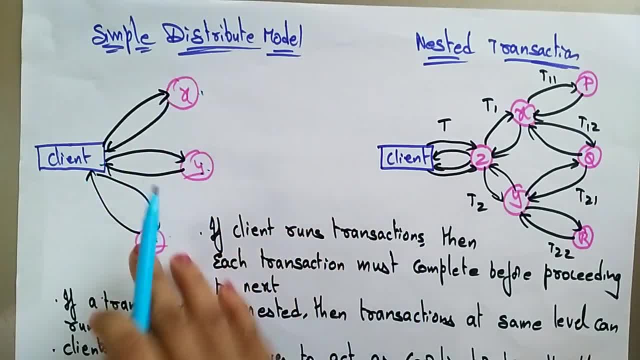 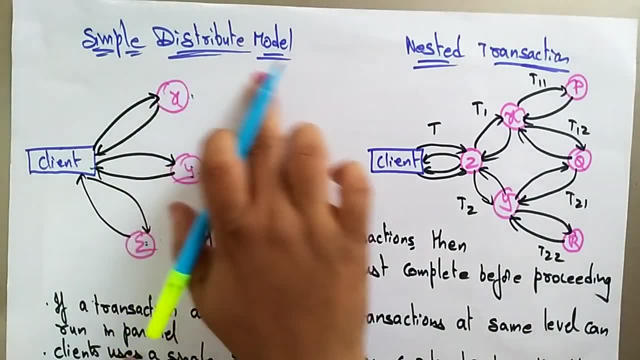 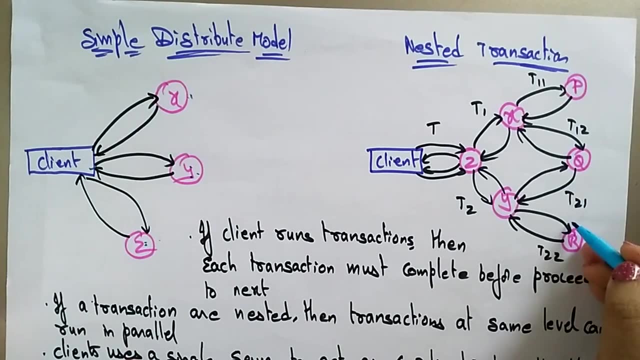 participants are there, so everyone is communicating in the distributed environment if you are taking the nested, not a simple three things. so these transaction again. these process again communicate with another process. these process again communicated with another one or two process, one or more process. so this technique you call it as a transaction. so here we have to allow the time. 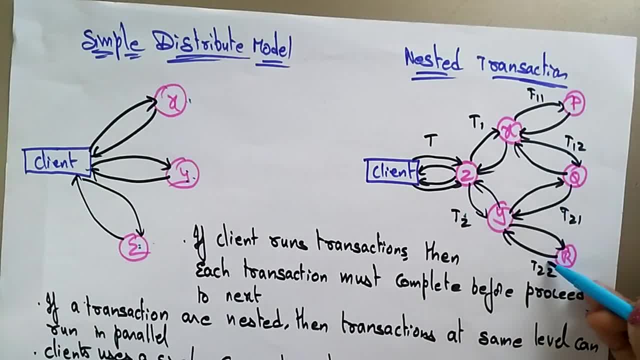 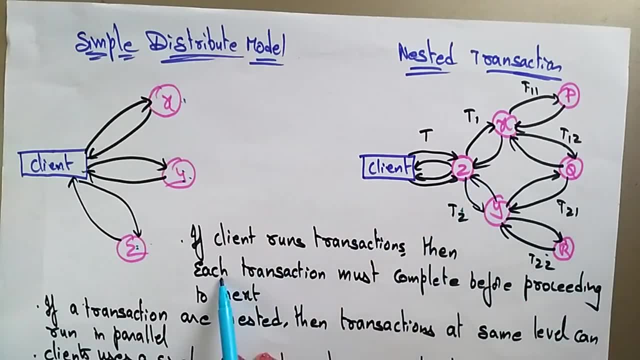 like t1, t2, t1, 1, t1, 2, t2, 1, t2, 2, like that. so here, if clients runs transaction, if client runs transaction, then each transaction must complete before proceeding to the next. so the thing that you had. that's why we are assigning the numbers to the transaction, so that we can recognized. 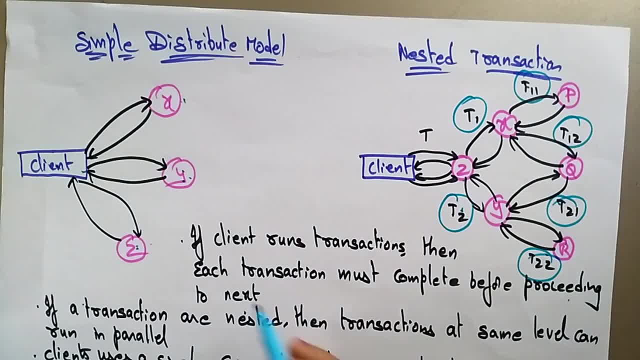 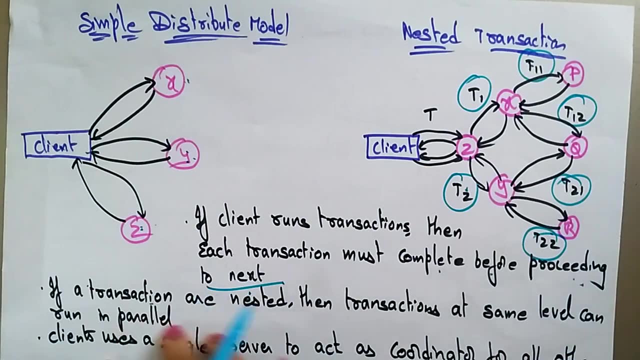 which transaction is running at present. so each transaction the client has to check. each has transaction must complete before proceeding to the next. suppose if a transactions are nested. if you taking this, if the transactions are nested, then transactions at the same level can run in parallel, so the transactions at the same level can be run. 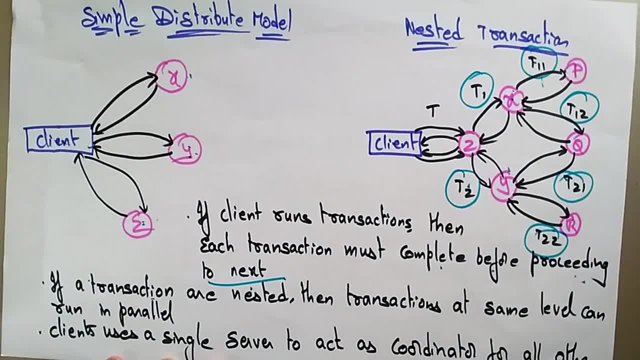 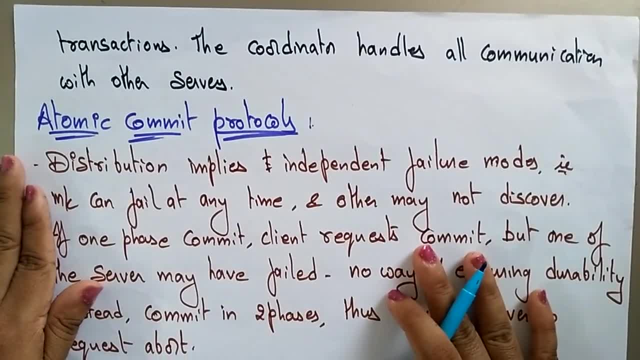 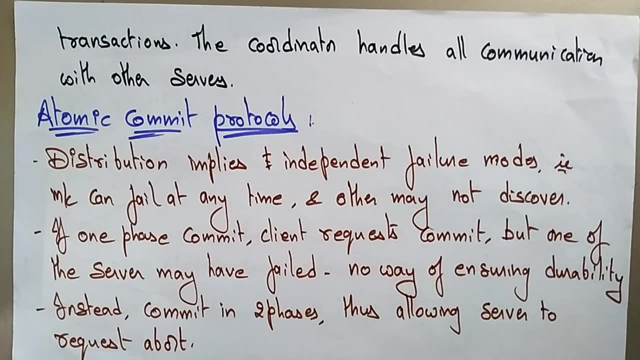 in parallel. here the clients uses a single server to act as a coordinator for all other transaction. so the coordinator handles all communications with other servers. now let me explain you some atomic commit protocols that are used in the distributed transaction transactions. okay, so in the distributed transactions the atomic more commitment. 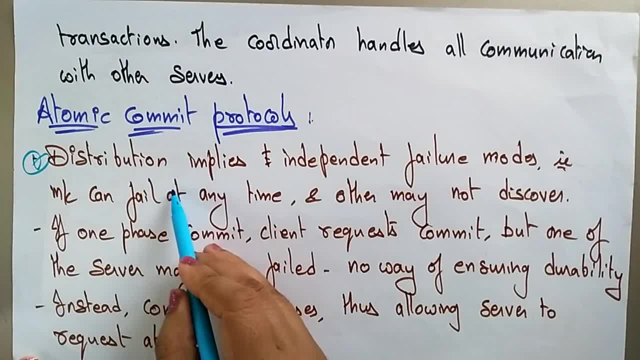 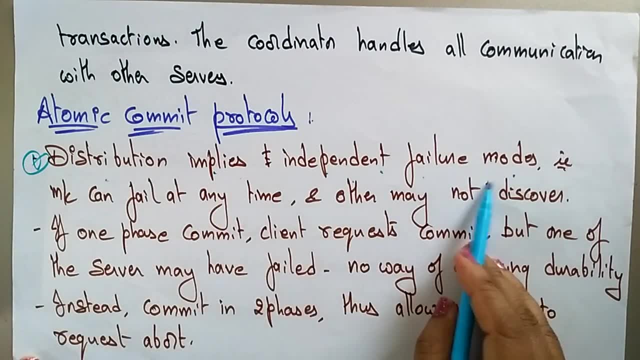 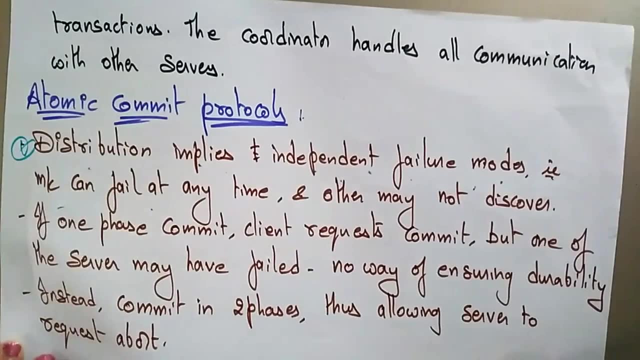 protocols are: first, the distribution implies independent failure mode. so that is the first thing. but ever we discussed, the distribution implies independent failure modes. that is, the machine can fail at any time and other may not discover it. so this is one of the problem. if one phase commitment, if you use the one-phase commit protocol here, the client requests the. 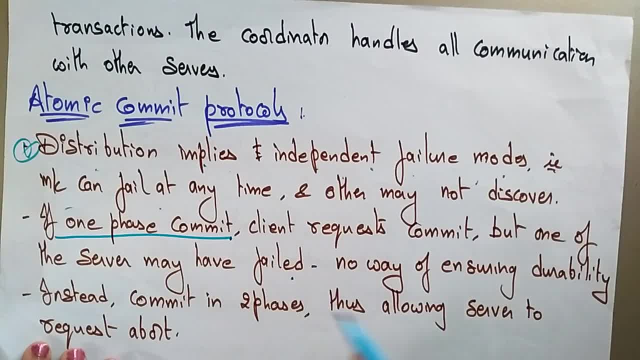 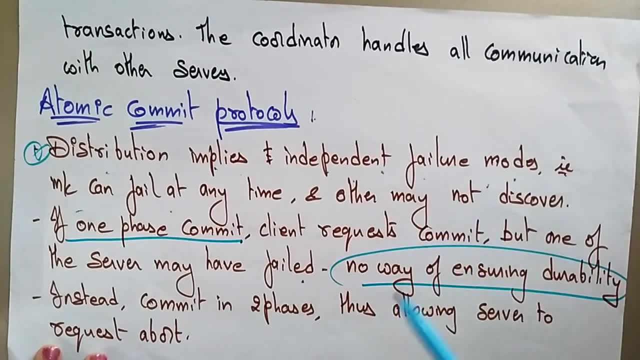 commit but one of the server may have failed, then no way of ensuring durability. so there is a main disadvantage in one-phase commit. so to overcome this one-phase commit, we are going to the two-phase commit. so what is the disadvantage in one-phase commit? if the client is requesting commit to the 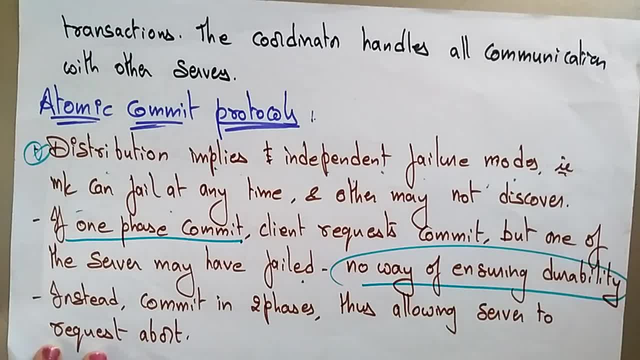 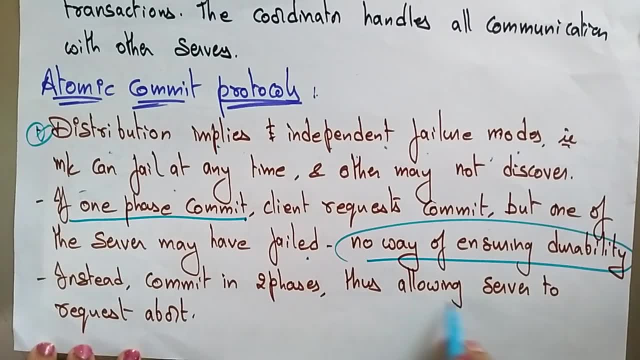 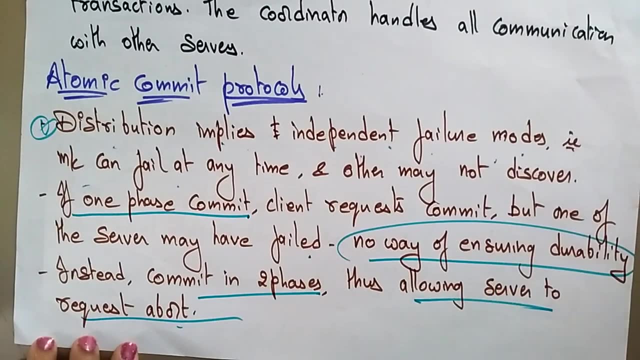 server. so before reaching that or sending the reply, the server has failed so there is no way of ensuring durability. instead, the commit in two-phase, thus allowing the server to request abort. so in the two-phase protocol, suppose when the server is going to be failed, the server has an ability to allow the request abort. it is simply sending the message request.